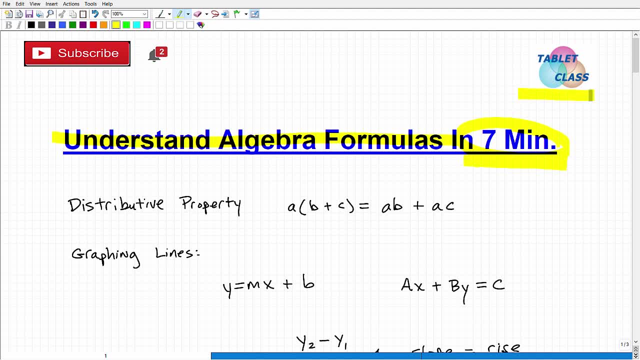 is John. I'm the founder of Tablet Class Math. I'm also a middle and high school math teacher, So I've been teaching algebra for decades. I've been teaching algebra for a long time, So I definitely know what I'm talking about And I actually offer a very, very comprehensive 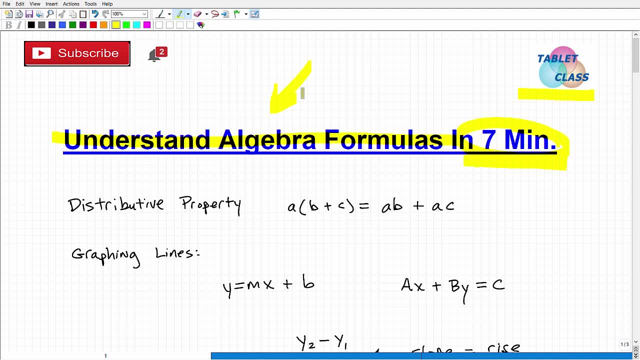 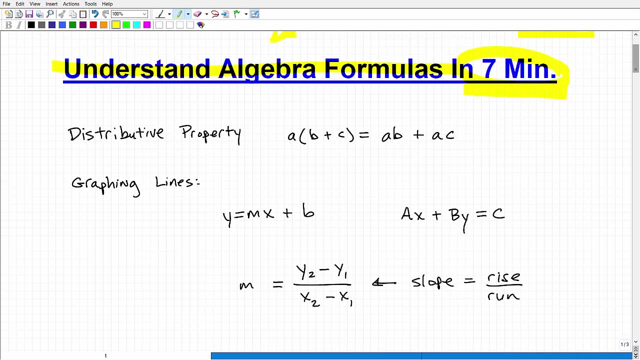 algebra course and other courses as well, Online courses. I'm going to leave a link to my algebra course in the description of this video. If you really want to get into, you know not just these formulas but the whole entire subject of algebra. Okay, so let's get right into it Again. I'm not 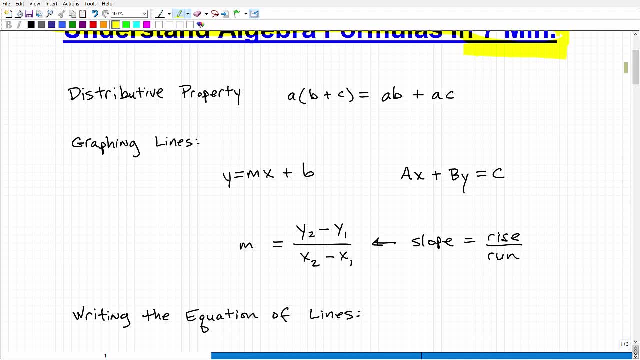 going to teach all these formulas, because I got a lot to kind of cover And I've broke these formulas down in terms of kind of in the order of how they would likely be presented to you when you take algebra. In other words, some formulas you're going to learn on in the beginning. 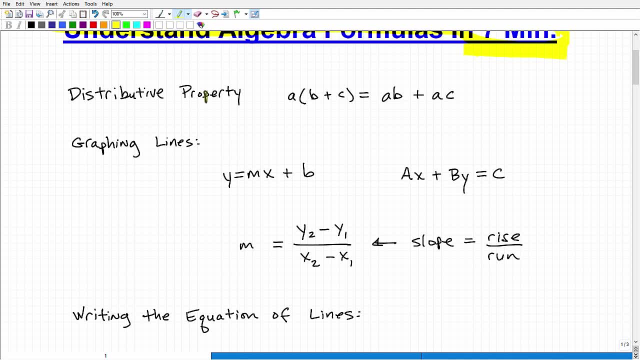 of the class and then in the middle of the class and then towards the end, because you know, math does build upon itself. Okay, so let's go ahead and get started. So the first thing I want to go and highlight is the distributive property. Again, there's. are there other properties? 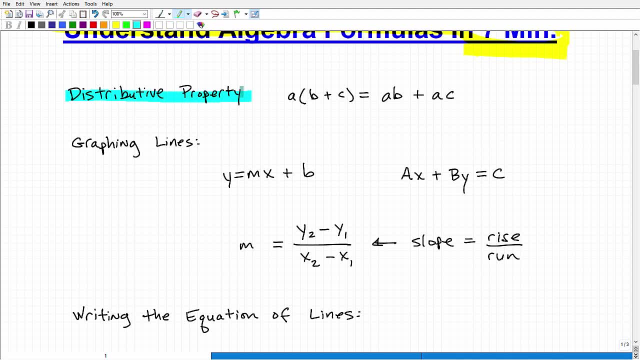 and there's other formulas, not going to write down every single one of them. This is an extremely important formula to remember in algebra. So it's the distributive property, And here it is. So it's a times b plus c equals a b plus a c. let's go ahead and just do a real. 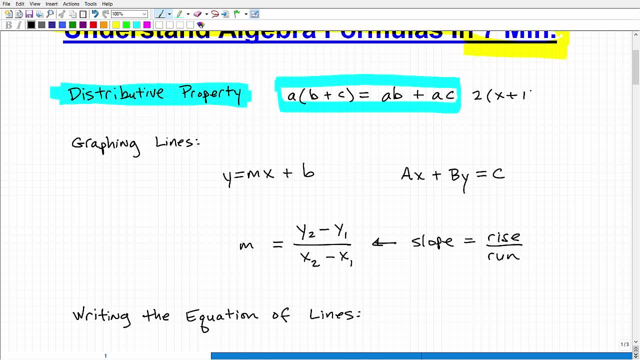 fast example. So it would be something like this: 2x plus one, if I'm following the formula. okay, just look to see where things are at what place. Okay, this would be a, this would be b, this would be c two times. 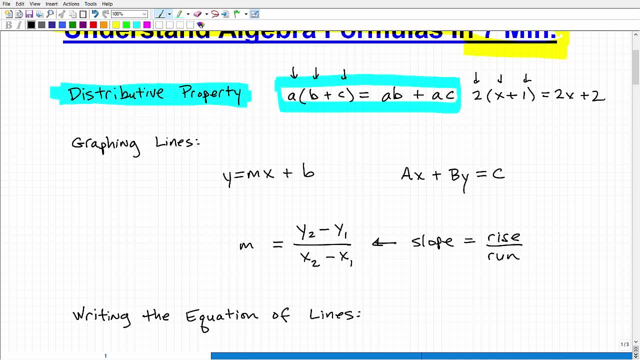 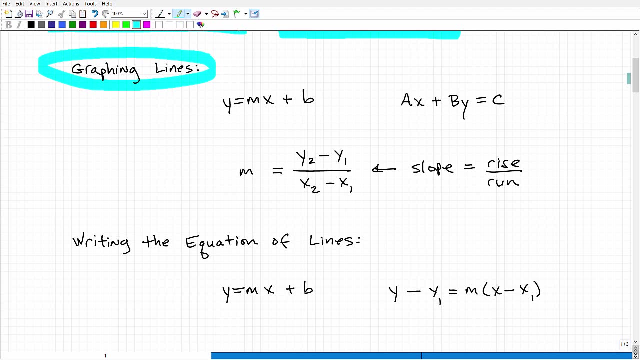 x plus one is the same thing as 2x plus two. Okay, All right, super critical property. make sure you know it. Okay, let's talk about the topic of graphing lines, or linear equations- big, big topic in algebra. So some of the key formulas you really need to understand is this one here: Okay, 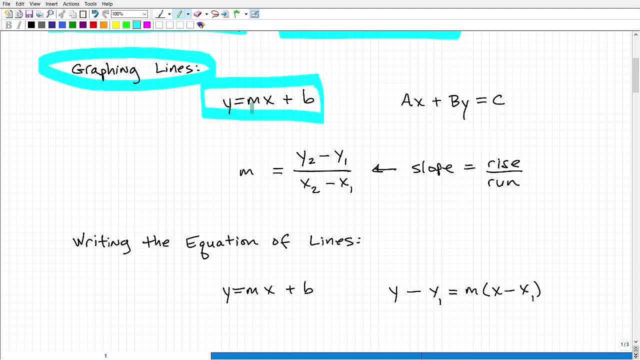 this is what we call the slope intercept formula of y equals m, x plus b. you definitely want to understand this, And this is when you would graph lines in standard form. So you use the x and y intercept here. So these are key formulas you need to understand when you're graphing lines. Now, along with that, you have 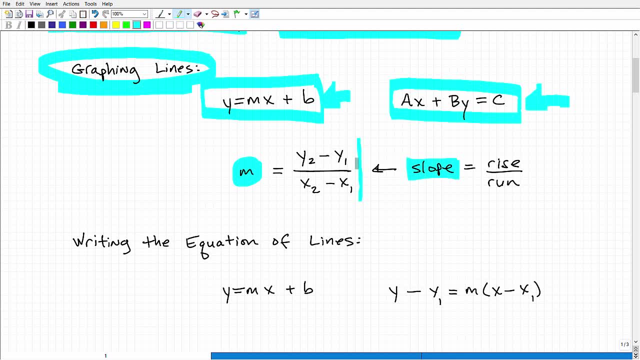 to understand the slope of a line. Okay, and this is the formula for the slope of a line, and the slope of the line is defined as the rise over the run. Okay, so when we're talking about the subject of graphing lines, these are key formulas that you want to remember. 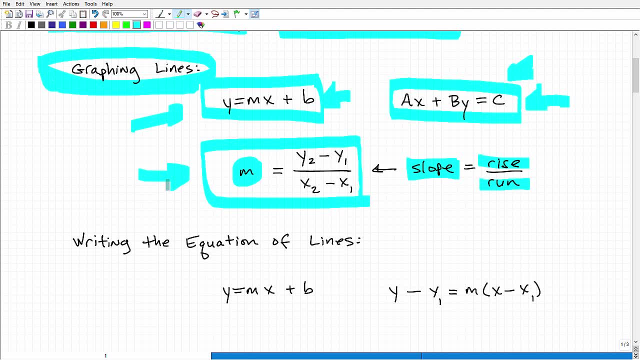 Now the formulas again, when I'm writing these- writing these formulas down- are formulas almost to the extent that you want to commit them to your long term memory. Okay, you're going to learn a lot of formulas and mathematics. Sometimes you're just going to put in your notes and reference them, But the ones that I'm kind of listing out here are things that you really want to try to you know, put into your long term memory such that you can reference them even without notes. That's why I'm kind of highlighting them in this particular video. 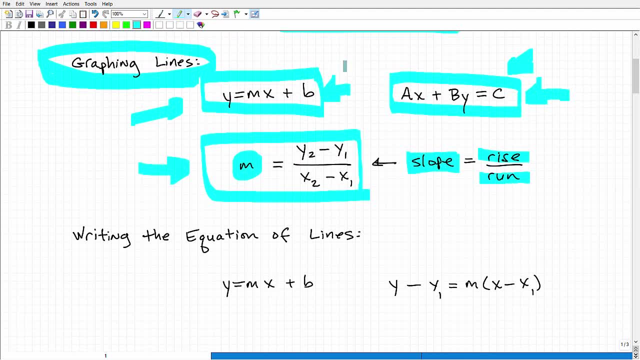 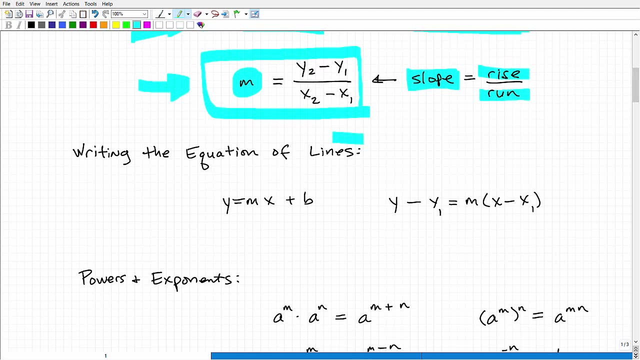 Okay, so once we learn how to graph lines- okay, we're given an equation like so And we go ahead and actually graph the line on x, y plane- then you want to learn how to write the equation of lines. So this is kind of the next step in algebra. So we're still going to use this slope intercept equation. And here is another formula- It's called the point slope formula- Super handy, very, very useful. You definitely need to know it. Okay, so these are two ways you can, two formulas you can use to write the equation. 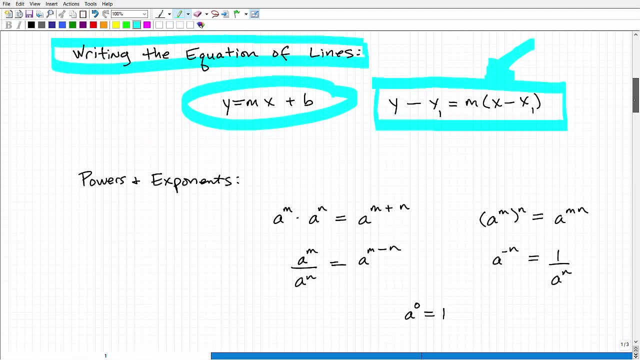 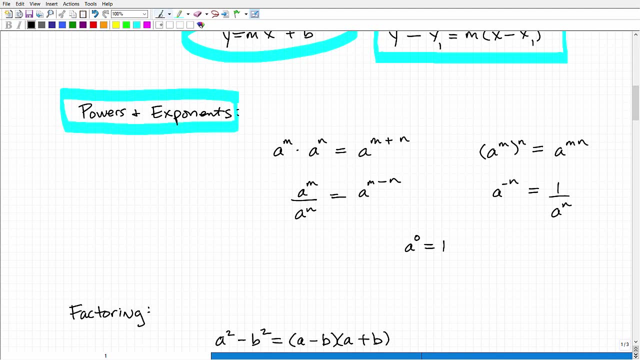 of a line in algebra. Okay. let's move on to another big topic in algebra And that's powers and exponents. You're working with- you know expression, something like this. let me go ahead and just write something here. Let's say: you had something like this, Okay, and you want to go ahead and simplify that. So you're working with powers and exponents- Again a huge, huge topic in algebra. 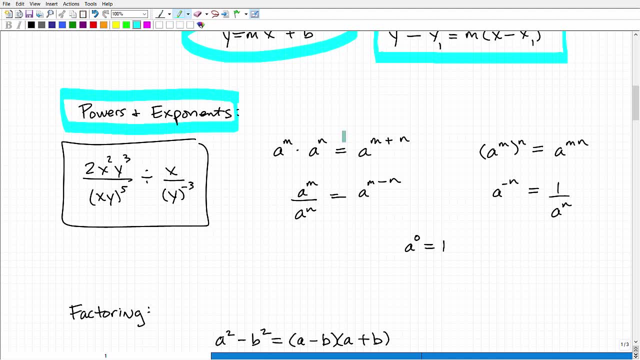 Okay, so there's different rules, different properties, And of course these are expressed as formulas. So here's our first one. this is called the product property. So a to the n power times a to the n power is equal to the a to the m plus n. Okay, so a down here. this is if they have the common base. So in other words, x squared times x to the fourth power, the x's are the same. In other words, the bases are the same. This is x to the 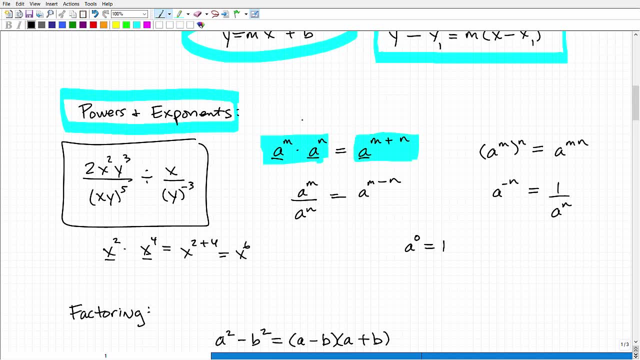 two plus four, or x to the six- that would be an example of this particular property. and then you have the division of powers. okay, and this is the formula for that. now, I'm obviously not trying to teach you algebra in seven to ten minutes. that's kind of crazy. but I am again highlighting the 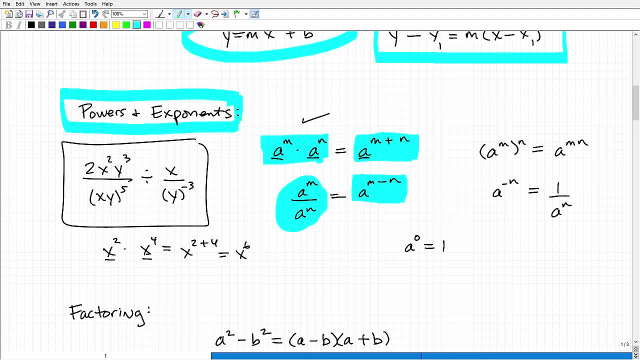 main formulas that you need to understand and kind of breaking them out or organizing them in the respective topics that you're going to see in algebra, okay, so you're going to have to know these here. you're also going to have to know this formula: a to the m to the n, power is equal to a to. 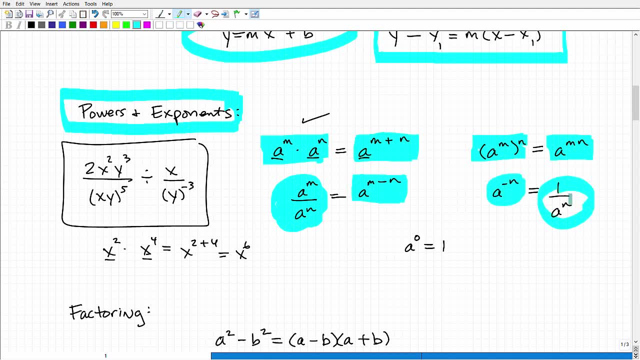 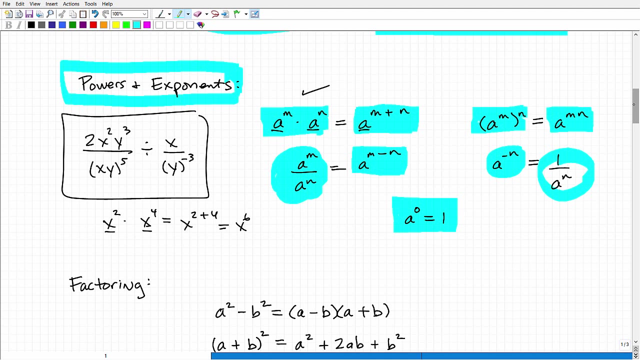 the m to the n, a to the negative, n is equal to one over a to the n, and then a to the zero or anything to the zero, power is one. okay, so let's keep moving forward here. now let me just make another comment. you know, obviously I'm going fast and some of you are like: can you explain this more? 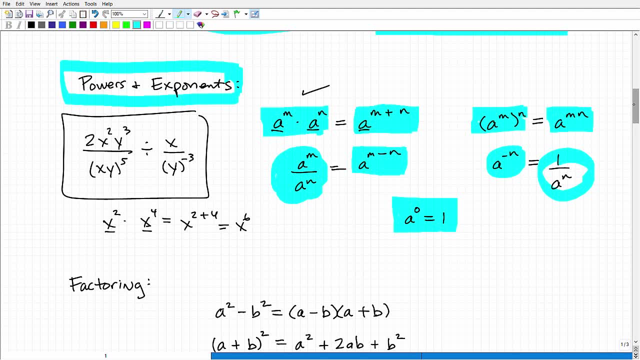 that's. that's for a different- uh you know um lesson, different video series. okay for me to go through this. this is a chapter. each thing I'm talking about here is like one full chapter in algebra. so if you really truly are struggling, you need to learn anything that I'm kind of talking about. and, by the way, this is not even 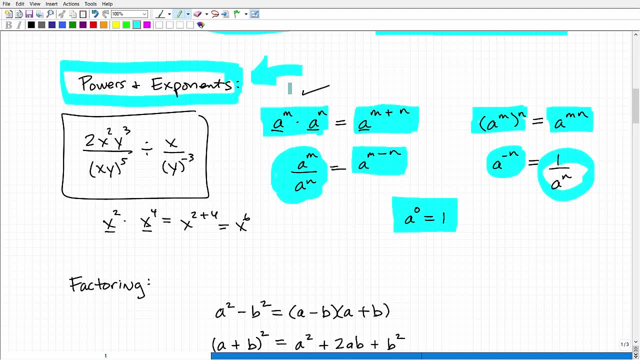 covering all the topics in algebra. there's other things like systems of equations, absolute value, inequality- that don't really have particular formulas to them. okay, so I'm highlighting again algebra that uh are key, okay, but it doesn't mean that it's going to cover all the topics. 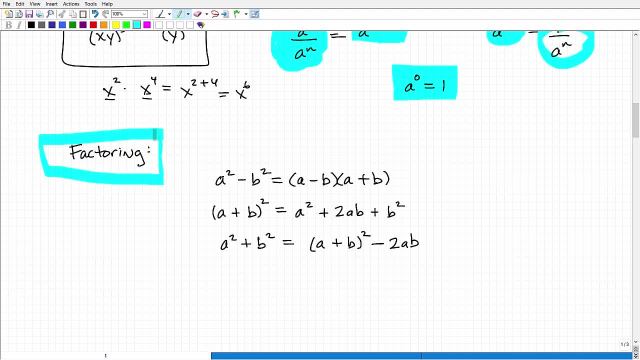 all right, let's talk about factoring. okay, so factoring polynomials: here we have the difference of two squares. okay, it's expressed like so: so if we have something like this- x squared minus y squared, and we want to factor it, we can follow the difference of two squares formula and we can. 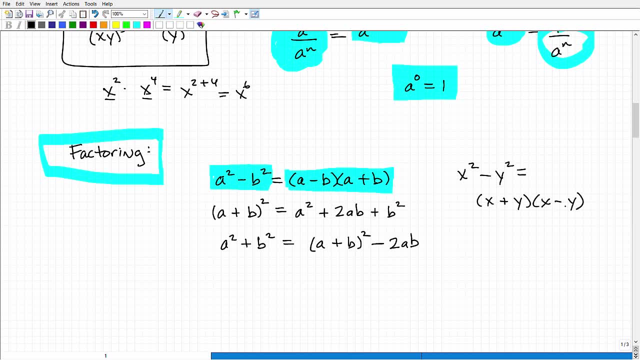 write it like so: x plus y times x minus y. factoring is so important. everything is critical, but factoring is one of these skills that if you can't factor, you're not going to be able to do so many other uh chapters and sections in algebra. 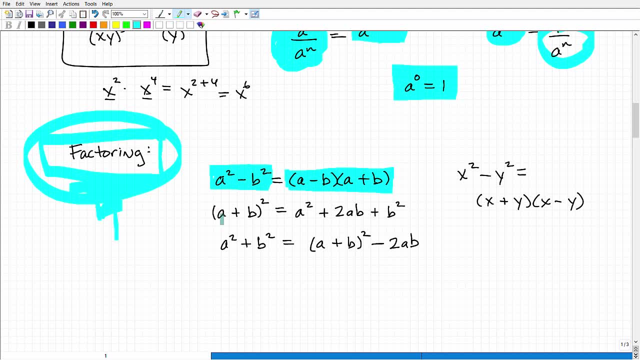 so if you don't get factoring down, you're really going to have big problems. but these are some key formulas here for factors. there's other formulas, but these are some ones that you really, you know, want to commit, kind of the fundamental ones that you want to commit to memory. okay, so factoring: 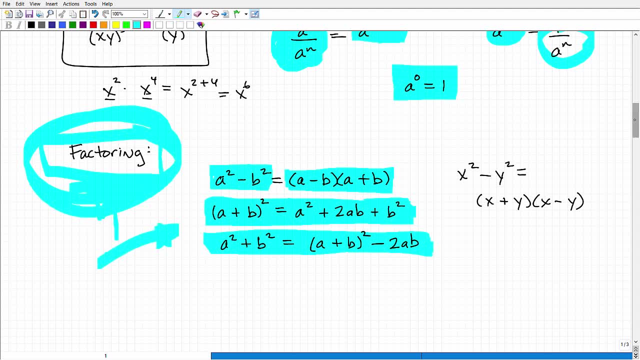 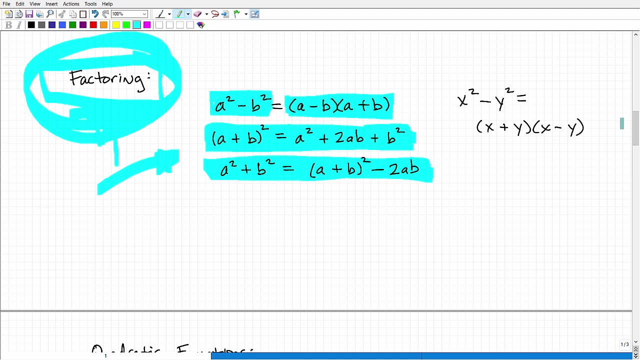 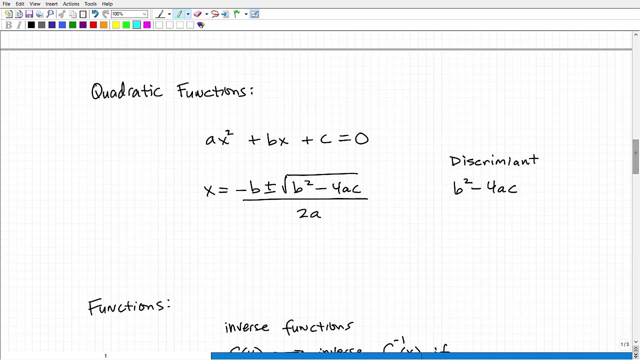 formulas really, really critically important. okay, let's just keep this moving again. uh, if you're struggling with anything you're like, oh, can you explain this? just go to my algebra link in the description of this video and you'll learn more than you'll. you'll learn a lot. okay, you'll master this stuff. 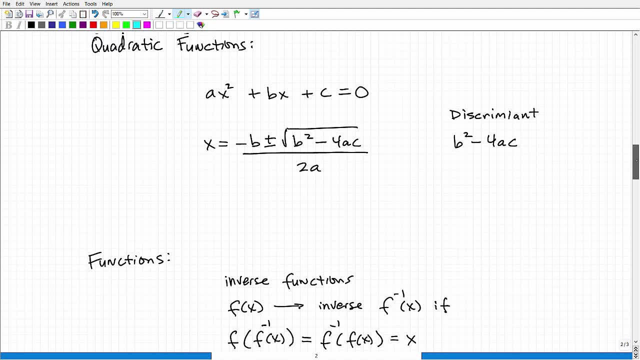 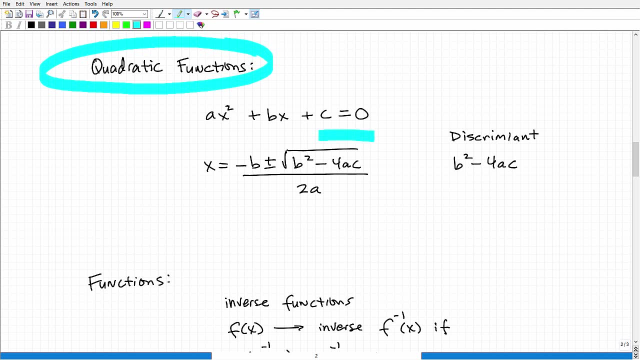 I'll teach you from the basics to the, to the advanced stuff. okay, let's talk about quadratic functions or quadratic equations. so the two big, the biggest formula is the quadratic formula. okay, this is critical. so, given a quadratic function expressed in this manner: a to the x square plus b, 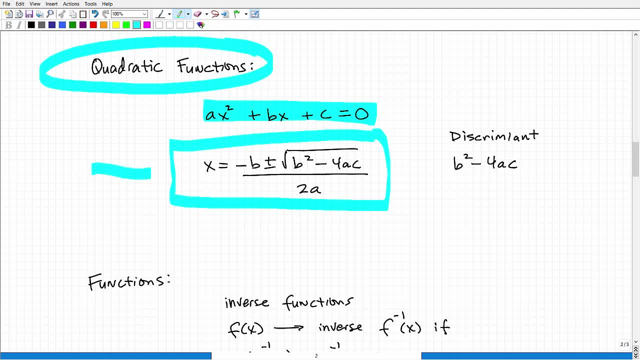 times x plus c equals zero. okay, this is how we find the solutions to this particular quadratic equation. in this manner, you only want to use this quadratic formula when you can't solve this using other, simpler ways like factoring or taking the square root of both sides. 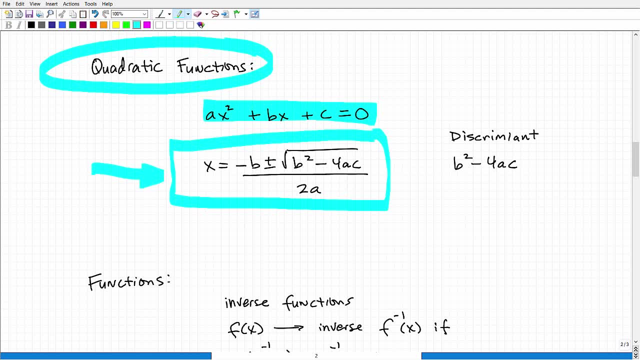 but if you can't do any of that, you have to use a quadratic formula, and this is something I would definitely commit to your long-term memory. for sure, You definitely need to know how to use it, But beyond that, you know, I would commit that to your memory. 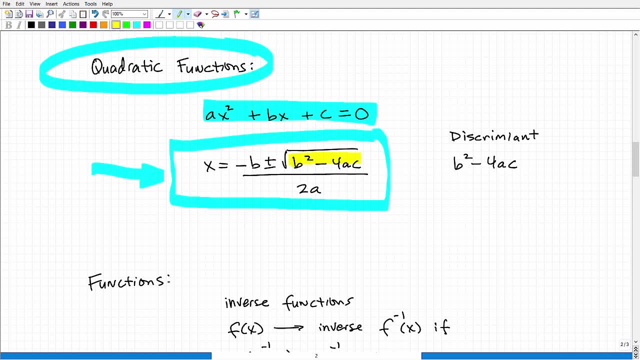 Now this part here of the quadratic formula, this is called the discriminant- okay, And this is going to basically determine the type of roots, type of solutions we're going to have for a quadratic equation. okay, So there's always two solutions to a quadratic equation. 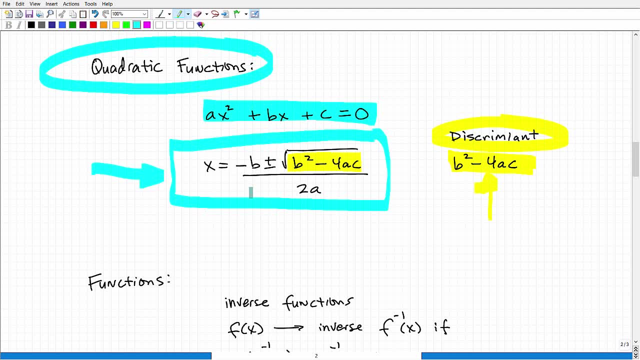 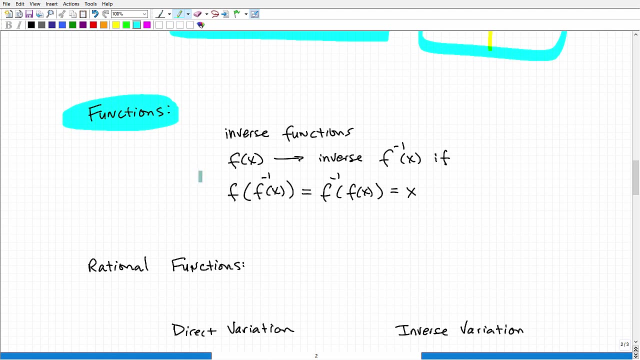 You can have real number roots, or you can have complex or imaginary number roots. The discriminant helps us determine what type of roots we're going to be looking at. Okay, let's move on to the topic of functions Now, another huge topic in algebra. 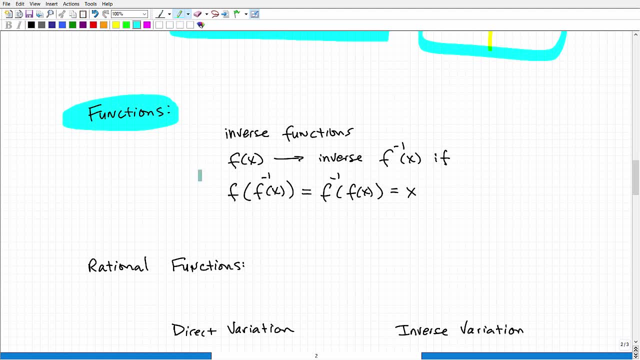 I wouldn't say there's so many formulas, but if I did have to think of one formula, there is a. when we're talking about inverse functions, the definition, The definition of an inverse. okay, if you're given a function, f of x and we want to find its inverse function, 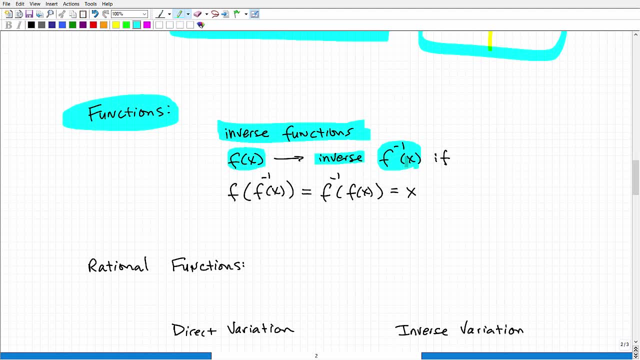 we would express that as f of negative, 1 of x. okay, So this is the inverse of this function. Now, they're only inverses of each other, if this formula holds true, okay, In other words, if you could take the composite function of both of those functions and the answer is just x, okay, 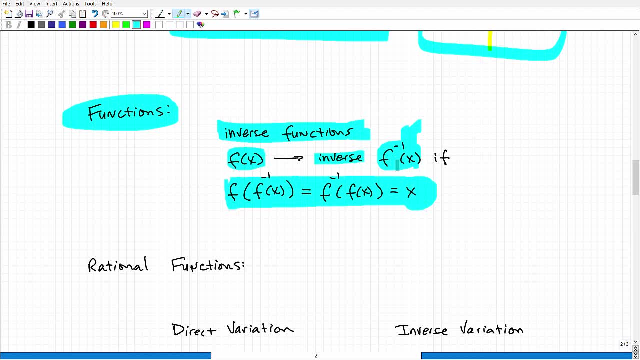 then in fact f of x is the inverse of x. So f of x and f of negative 1 of x are indeed inverses of one another. So this is kind of a formula that you do follow when you're talking about functions. 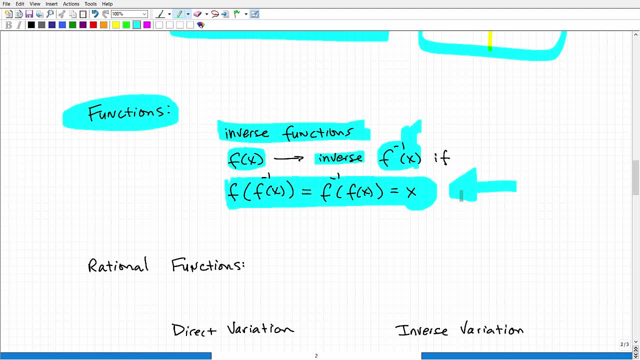 But again, a huge topic, but not really like formulas, like the quadratic formula, et cetera. You know a lot of these topics. you're not going to, you know have to. you're going to need to learn the concepts. 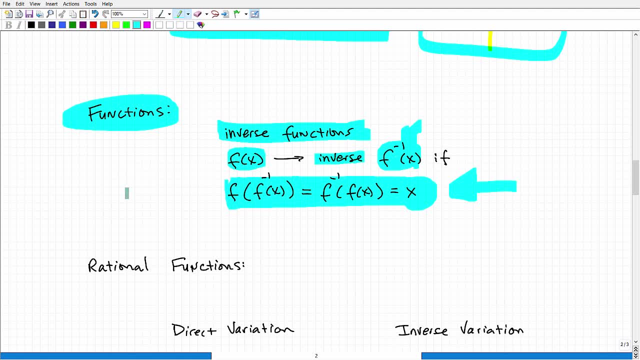 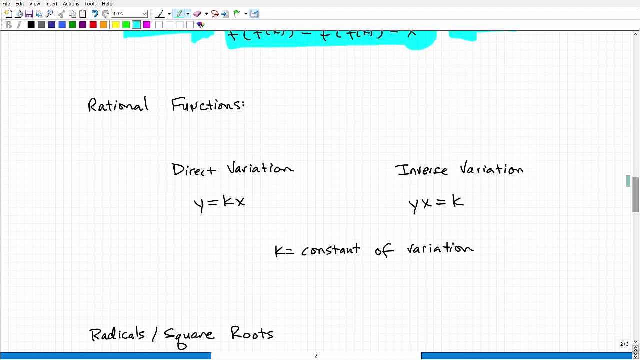 not to, you know, memorize some formula. But again, in the topic of functions, this is one particular formula that I can think of. that's critical. Okay, let's go down and talk. Let's talk about rational functions. This would include topics like percent, solving rational equations, big, big stuff. 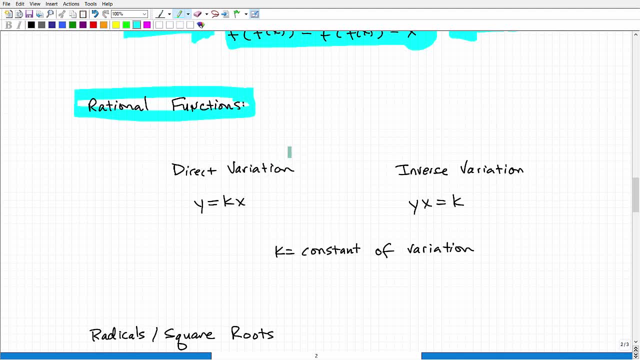 But in there, more often than not, algebra courses will teach the concept of variation And there's direct and inverse variation And the formulas for these are very, very important. So y equals kx is the formula for direct variation, And yx equals k is the formula for inverse variation. 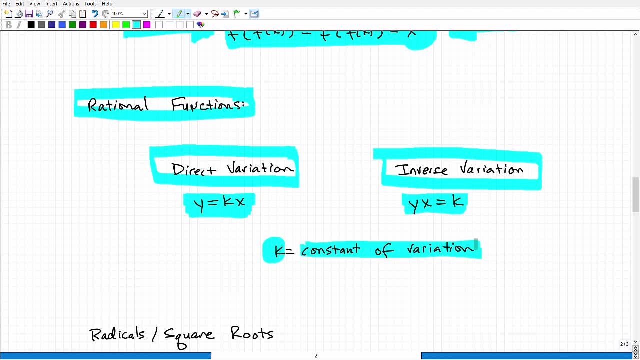 And this k is what We call the constant of variation. Now, one thing I want to mention is that I'm writing these formulas in this manner. It's probably the most common way you're going to see these formulas written, So your textbook or your teacher might express them. you know, using different variables. 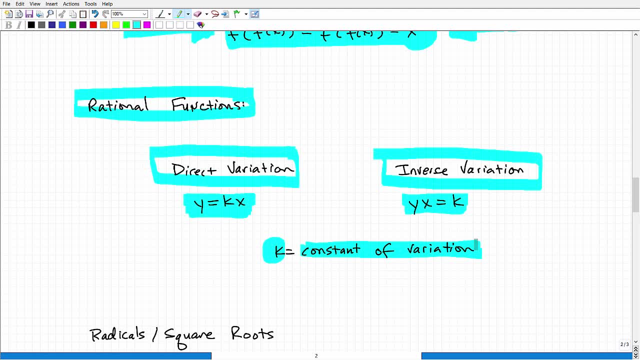 but likely, they're going to be using these same variables, Okay, but conceptually speaking, okay, the formulas are still going to be the same, All right. So, again, if your textbook uses ABC or some other textbook different- you know letters, you know variables- then just you know again. 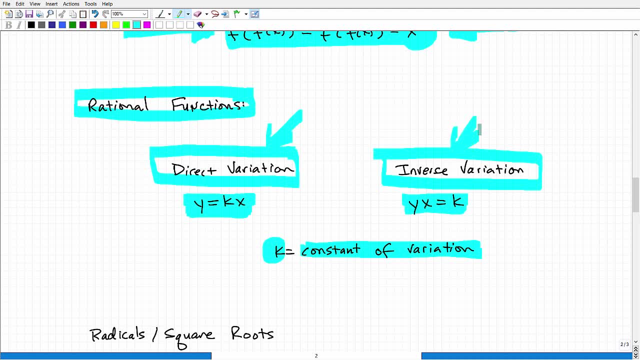 you still need to know the formula for direct and inverse variation at the algebra level, And the algebra level I'm talking about here is like ninth grade algebra, high school level algebra- Okay, not pre-algebra. Some of this stuff is pre-algebra. 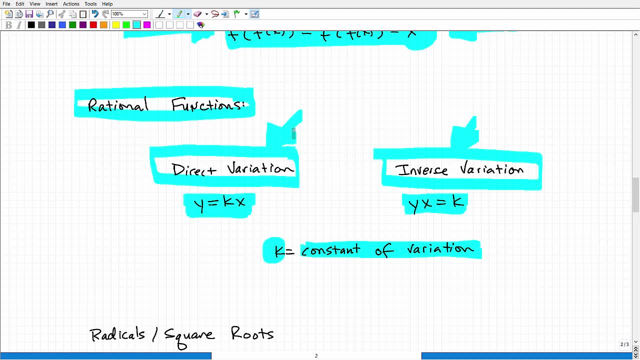 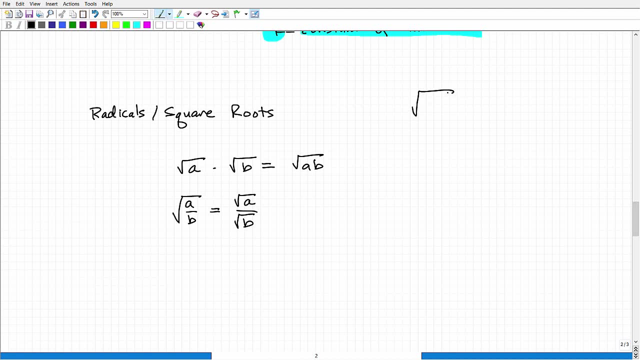 This is mostly like first year real algebra, high school level algebra. Okay. let's talk about radicals. Okay, and a radical is this thing? Okay, Okay. most people will say, oh, that's the square root symbol. Yeah, that's a square root symbol. 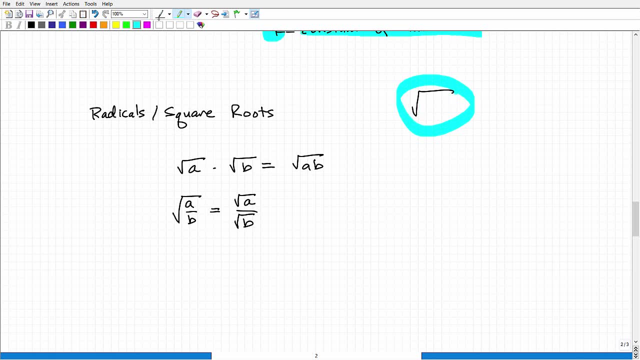 But technically, in mathematics, this is what we call a radical, because this is a square root by itself. But if I go like this, I put a little three up there. This is a cube root. A cube root is different than a square root. 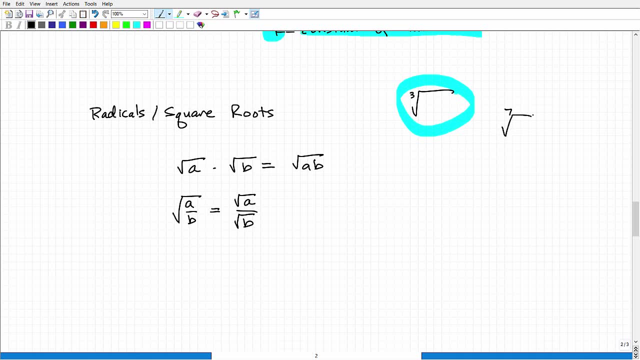 If I say like the seventh root, that's totally different than a square root. So this symbol here is a radical, But without any numbers here this is technically a two But two when we talk about a square root, but that's a radical. 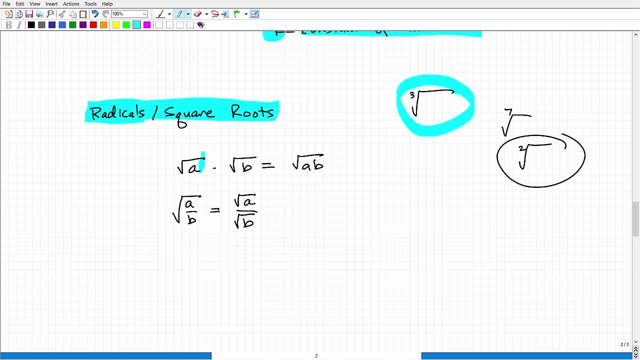 So under radicals and square roots- this is really really important, these formulas here. So the square root of A times the square root of B is equal to the square root of A times B. Okay, and then the square root of A over B is: we can break up this fraction as a square root of A divided by the square root of B. 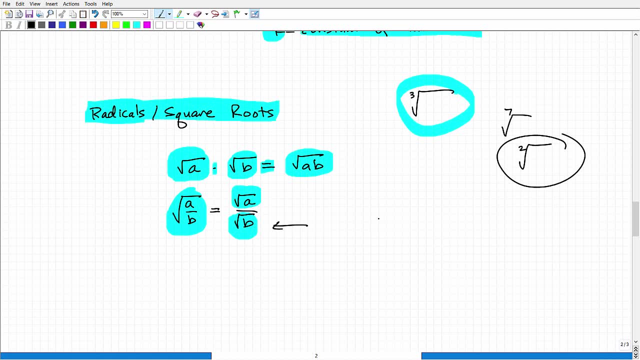 Now, when you get into a situation like this, okay, there's something. There's something called rationalizing the denominator. So, for example, if I have 5 over the square root of 3, okay, let's say, let me back this up here. 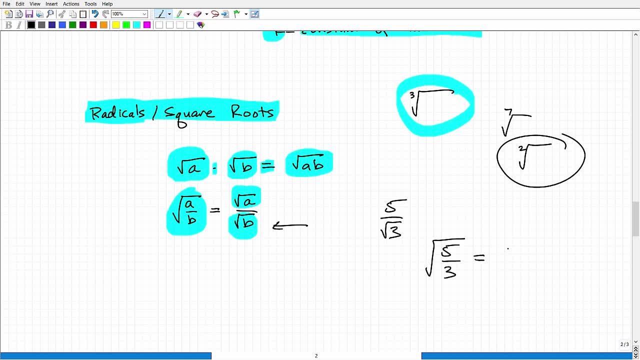 Let's say I had the square root of 5 over 3, and I write that as the square root of 5 over the square root of 3.. I'm allowed to do that, But when I have a radical with, or have an expression with a radical square root, an irrational number in the denominator, 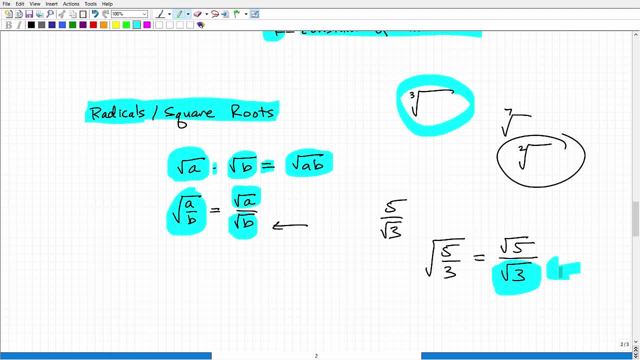 you have to do something called rationalizing. Rationalize That's not really like a formula, but it's something that you kind of want to, you know, be aware of, and certainly something you need to know in algebra. okay, I'm pretty sure I blew over seven minutes here, but hopefully you know, you can you know you're going to stick with me and learn this. 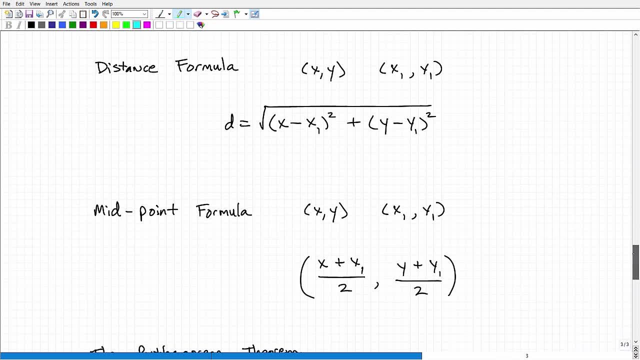 So let's keep going, Let's see, Do we have anything else? You have a few more here that I picked out: The distance formula, okay, really, really important. So let's say I have two points on. Okay, so here's x, here's y. I have some point here, some point there. one of those points is x- y, another point is x sub 1 and y sub 1.. 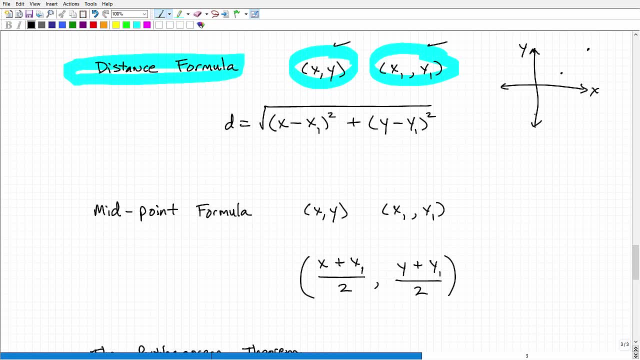 These are just two unique points on x- y plane. Okay, if I want to know the distance between those two points, I can use the distance formula. So this is the distance formula there, okay, so something you definitely need to know how to use, and the midpoint formula. 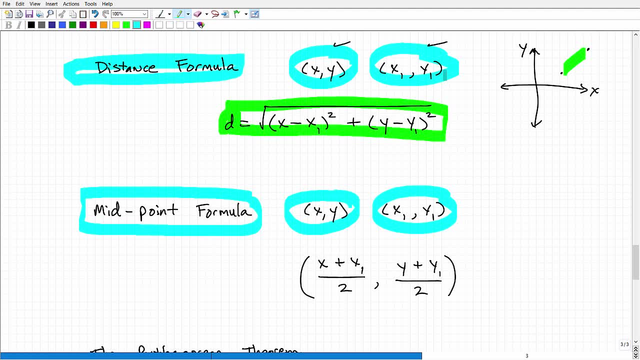 Now let's take these same two points. okay, if I want to know the midpoint- in other words, here's my two points- if I want to know the point that's in between, like exactly between those two, ie midway between this point and this point, that's the midpoint formula. I would use this formula here. 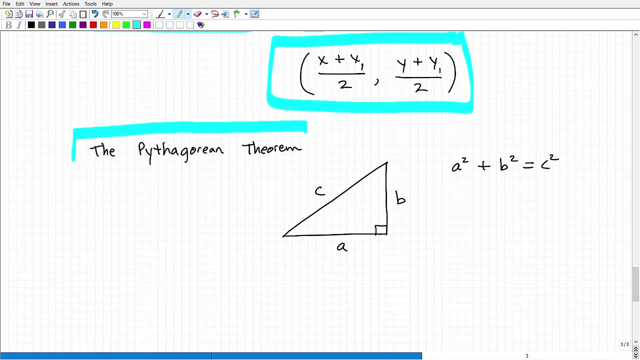 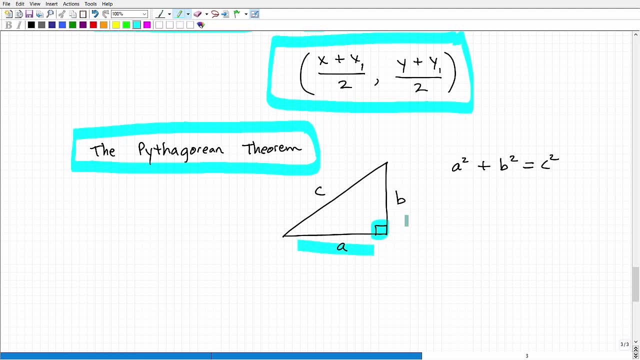 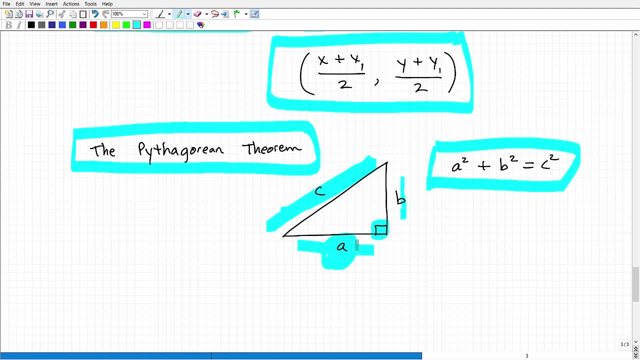 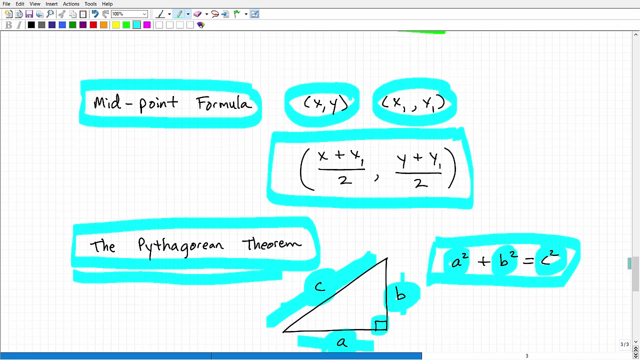 The Pythagorean theorem will hold true. So in other words, this side square plus this side square is always going to be equal to this side square. okay, Super critically important Pythagorean theorem. Of course this plays in geometry and trigonometry, etc. all this stuff here in algebra that i went over is, you know, maybe a. 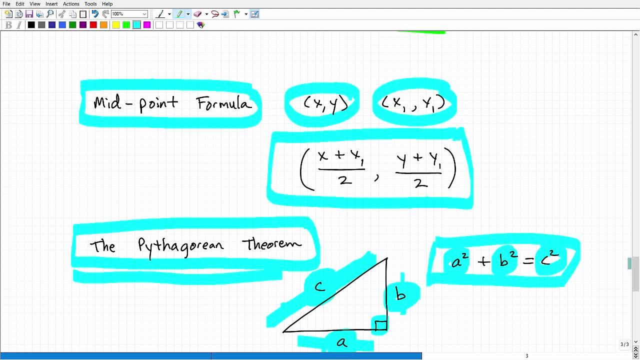 third of the topics. i mean, i'm just kind of hitting the surface in- and what would be covered in algebra? course we, even we didn't even talk about systems or inequalities or absolute values or, uh boy, other topics in there. so you know, algebra is a huge, huge, um, uh, course you know you're coming.